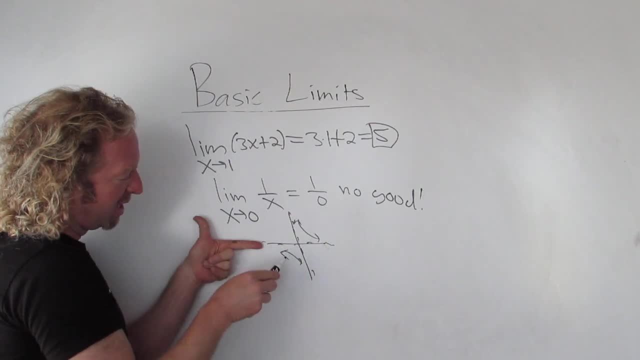 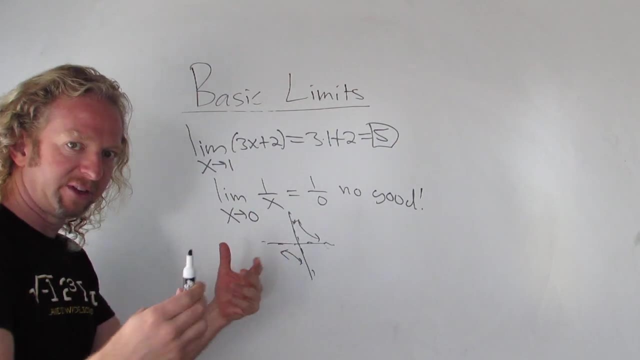 Therefore, you get different values, so the limit does not exist Again. as you approach 0 from the left, it goes down forever, so you get negative infinity. As you approach 0 from the right, it goes up forever, so you get infinity. 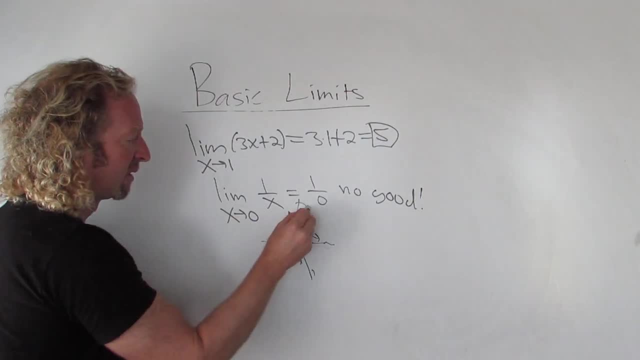 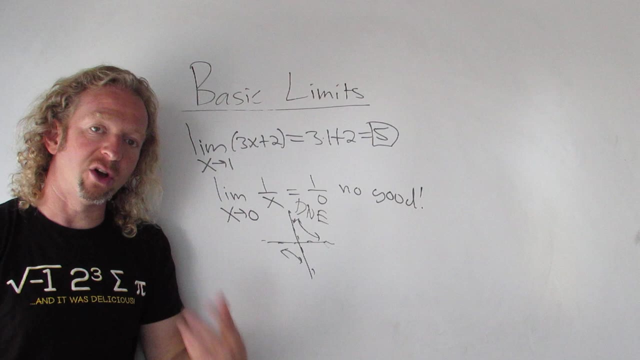 Infinity is not equal to negative infinity, so this limit is dn. There's not really a nice algebraic way to do this limit. Moral is: if you can plug in the number and you get an answer, you do it. If you don't get an answer, then you try something else. 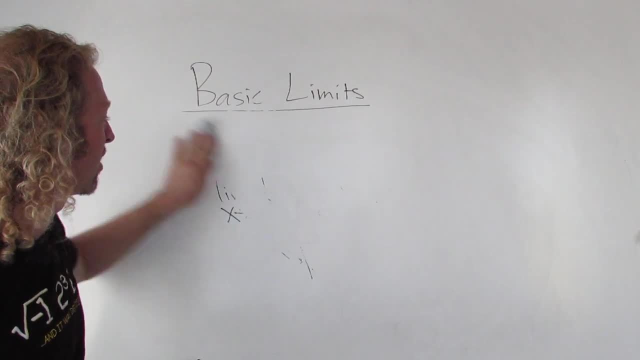 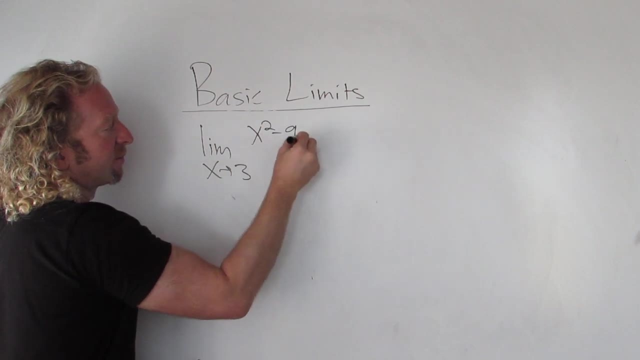 Let's do another example, just so you see what I mean. Let's try this one. Let's take the limit as x approaches 3 of x squared minus 9 over x minus 3.. So in this case, here, if you plug in 3, you would get 0 over 0, right. 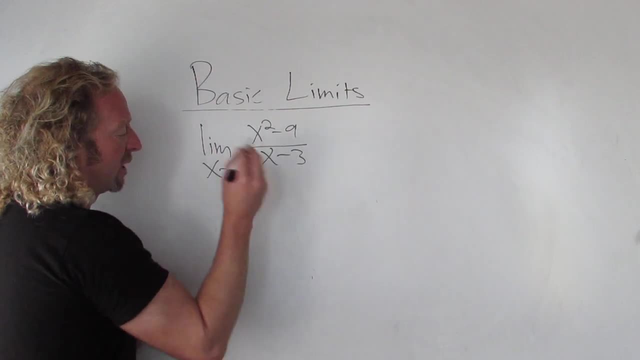 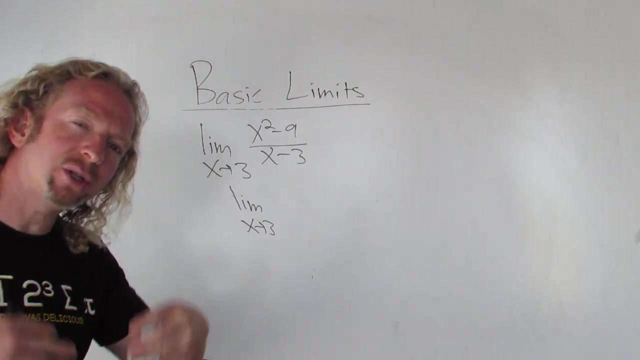 So that's no good right. So what do you do? Well, it looks like you can factor, So let the limit sign again. Now it's really important to always write the limit sign until you actually take the limit, okay. 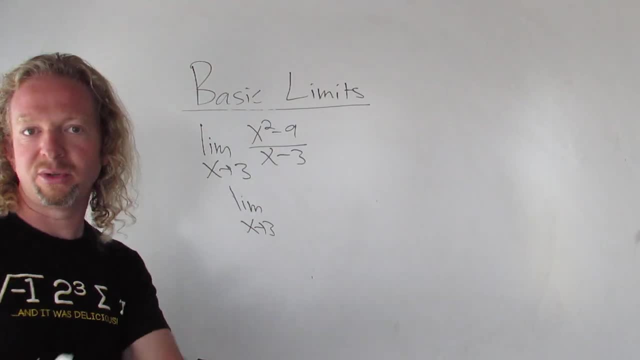 By taking the limit, I mean, like using a formula, plugging in a number, using you know some technique that gives you the result. In this case, we're not plugging in the number yet We're going to factor this right. 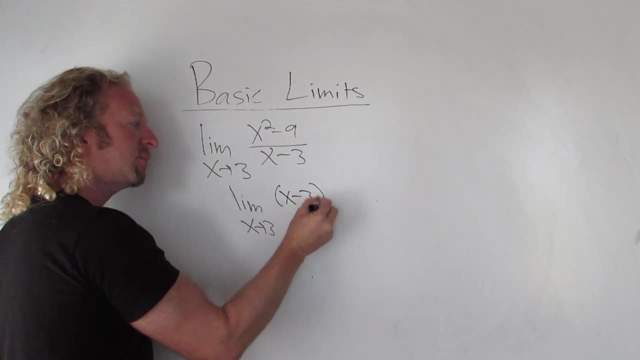 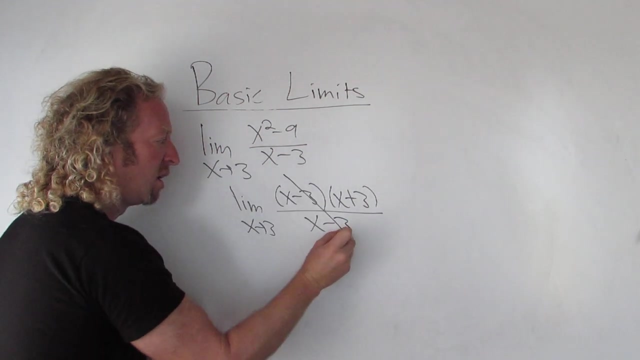 This is the difference of squares, So it'll be x minus 3,, x plus 3,, all over, x minus 3,. okay, Now you just cancel. We're not going to plug in the number yet, So I'll rewrite it one more time. 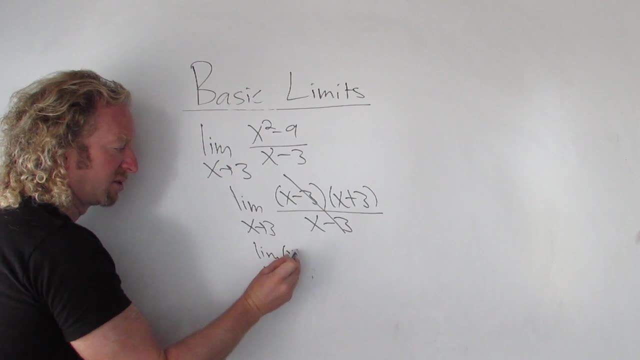 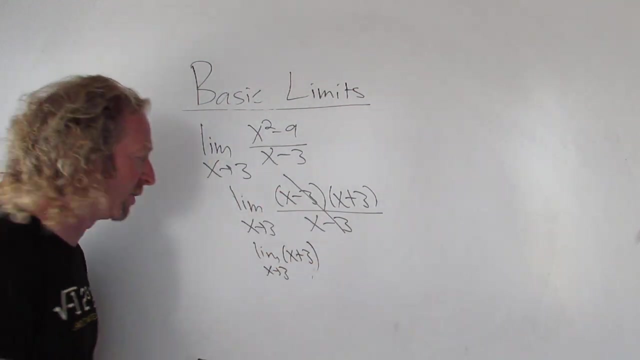 This is the limit as x approaches 3 of x plus 3.. So you always write the limit sign right, no matter what, until you take the limit. whatever that may be right, In this case taking the limit is plugging in the number. 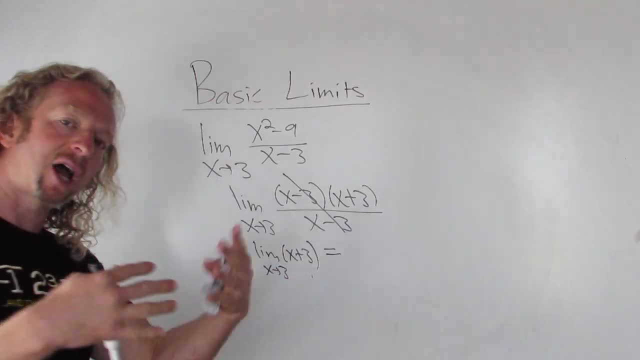 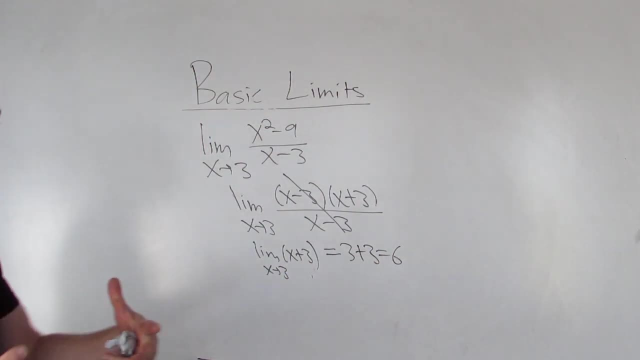 So we're going to take this 3 and put it there. When you plug in the number, that's when you stop writing the limit sign. Super important, right. So 3 plus 3, which is 6.. One of the most common pitfalls. one word to use in calculus. 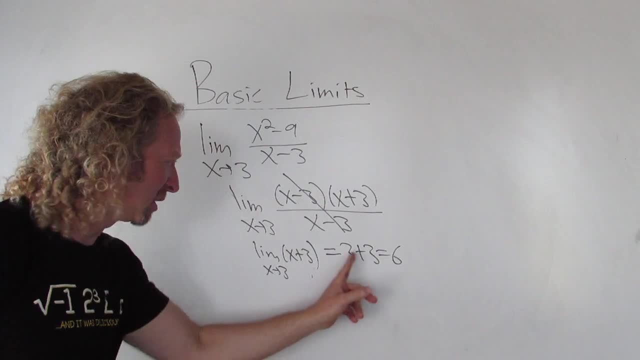 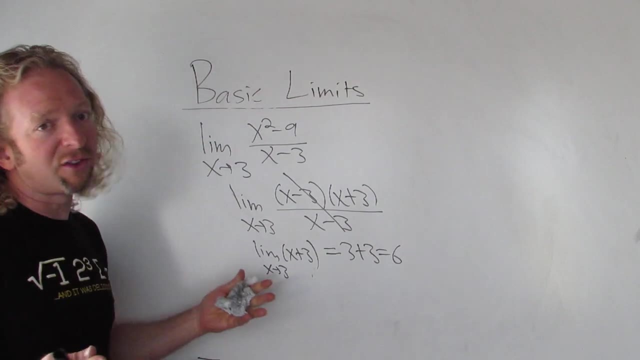 is people will drop the limit sign Or they'll put it where it's not necessary, Like if you put the limit sign here. that would be wrong, You've already taken the limit. So a lot of it is about structure in calculus and in all of mathematics. 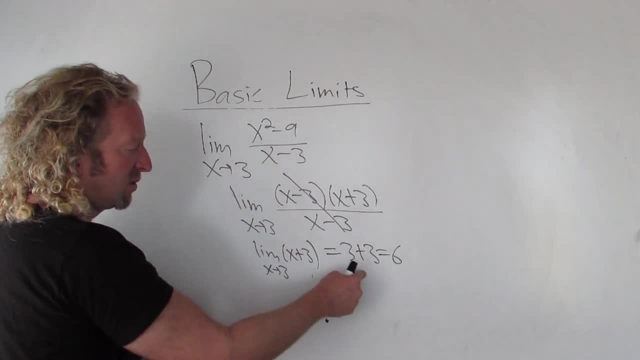 So again, the main rule in limits is: if you can plug in the number and you get an answer, do it. If you can't do something else, And what is that something else? Well, that's the rest of the course.